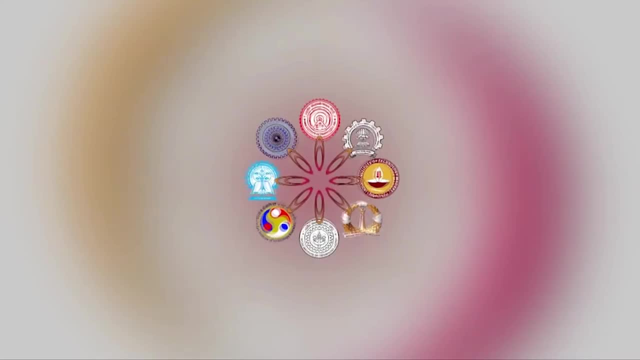 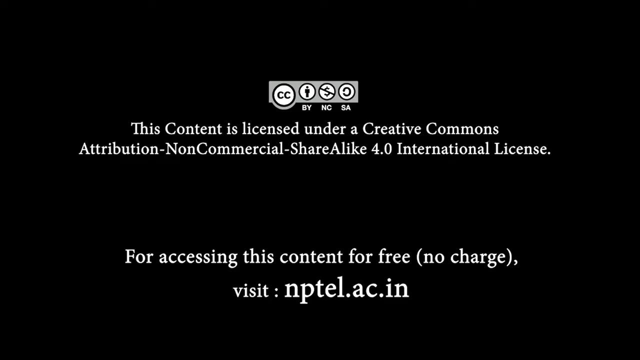 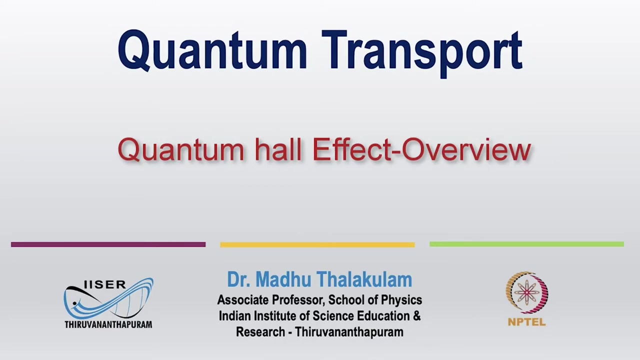 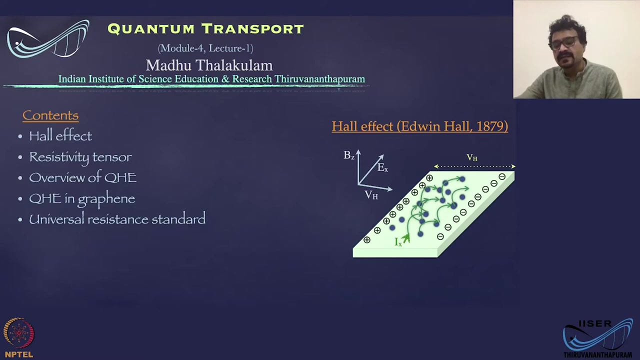 In this module we will start discussing a touchstone quantum phenomena or two-dimensional system, that is, the quantum Hall effect. So before we dwell into the details, let us quickly and briefly review the classical Hall effect, which was discovered by Edwin Hall in the 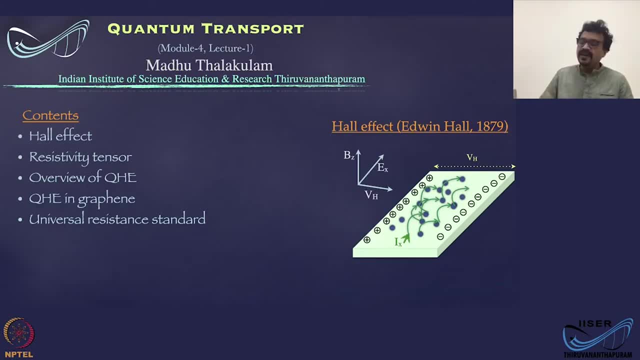 1980s, 1979.. So what you have here is you have a conducting material and you have a magnetic field which is supplied to the plane, normal to the plane, and you have an electric field along the plane of the sample And the transport of electron is driven by lot of. 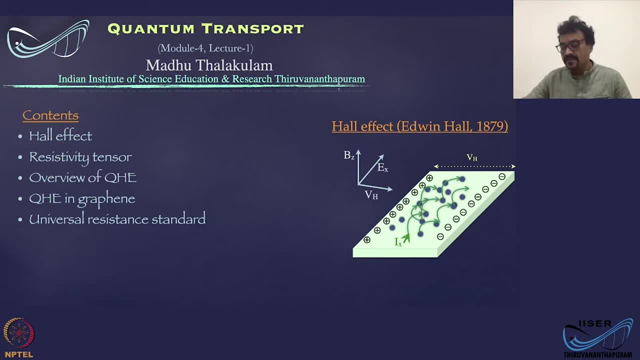 collision process as described by the two pictures, two spheres. Now the electrons will undergo cyclotron motion, but at the same time electron will undergo many collisions and eventually the electrons will get deflected towards one end of the one edge of the sample And other end you will have the positively charged ions. 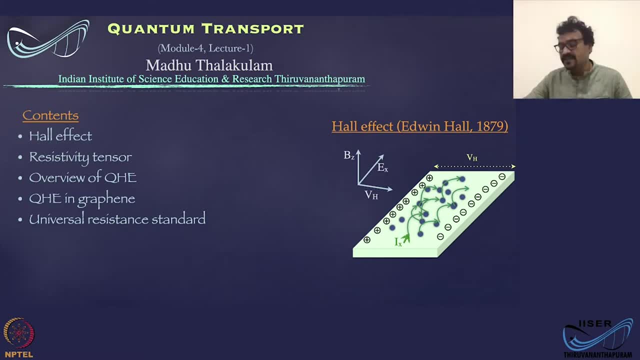 And at some point of time, a balance will be reached by the cyclotron motion. This is the cyclotron motion applied by the field, generated by the exposed ions and the collected electrons, and no more electrons will be actually collected and there will be a steady state where a voltage 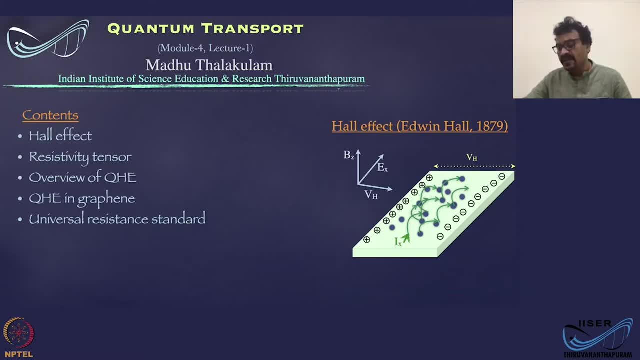 is generated across the edge, that is, the d, h, the whole voltage, and from this whole voltage we can get information on the k-ray consolidation in this, in the sample, and we can also extract other. from the k-ray consolidation we can extract mobility, conductivity and all these details. 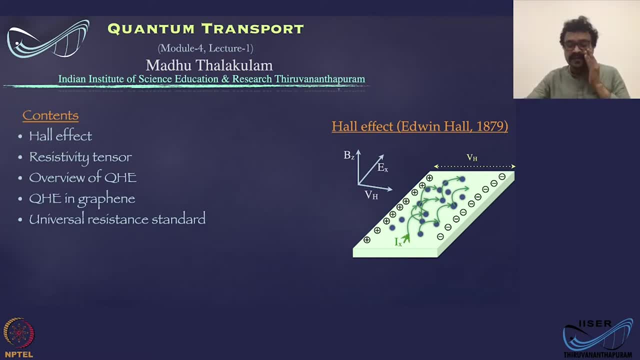 okay, now in this lecture we will briefly we will go through the mathematical formula, some of the quantum for the hall effect briefly. then we will define the sensitivity tensor and overview the quantum hall effect and we will look in the quantum hall effecting graphene and how the quantum hall effect is used as a universal persistence. 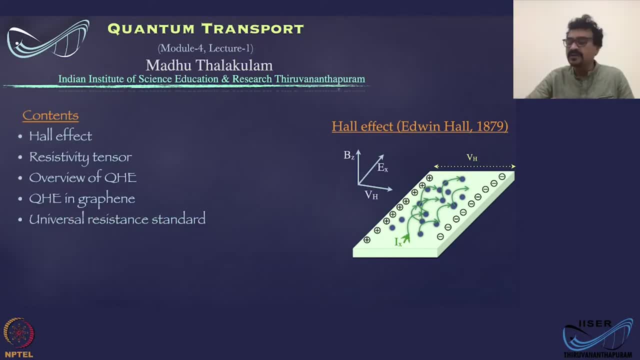 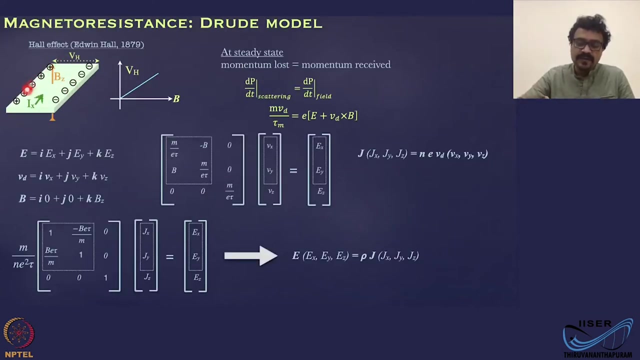 standard. so that is the plan for this lecture. okay, then next lecture we will look in the mathematical formalism of the quantum hall effect. now, how do? how are we getting the quantized persistence and all those details in the coming lectures? okay, all right. so this is the picture of the sample, where we have a magnetic field which is applied. 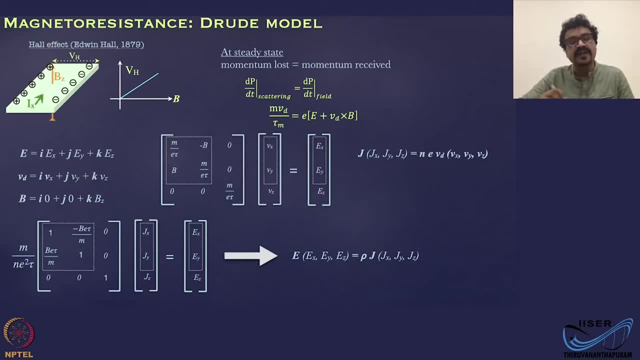 perpendicular and there is an electric field which is driving the current i x. okay, and the quantum hall effect actually is slightly different. that applies to a two-dimensional system, but in this case we we are considering it's a three-dimensional material. okay, the normal hall effect. what you have is you have a b field and you are plotting. 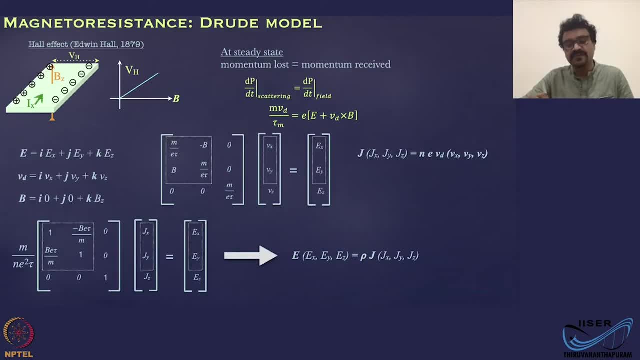 the whole voltage or the whole resistance. if you divide the whole voltage by the current, then you will get the whole resistance. then you will get a straight line, that is, the whole voltage is proportional to the b field. now the assumption here is the carrier constant, the carriers undergo. 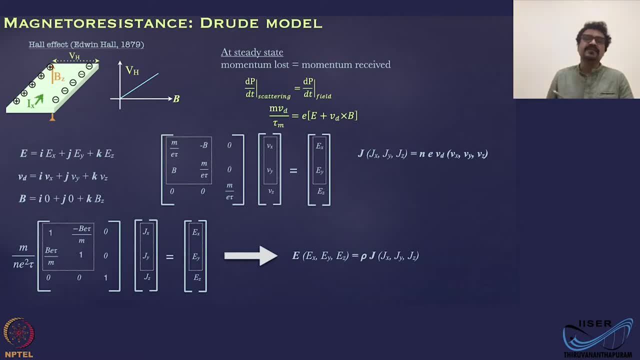 a moment on a random relations right. and if the colonies are incorporated and the birds coloured only as that state that you saw, please review it. if you, for example, still see in in dubbed attala lived, but if the creative Nazis and other psychologists can survived like quite a while but joining siebel, all, but it doesn't affect the value, okay, so this type of representing is a non- temos, drinking and значит. 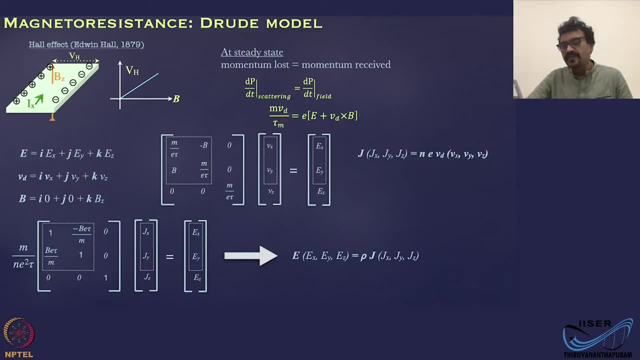 is the drift velocity, tau m is the scattering time, or that is the force experienced by the charge carriers. ok, And there is a force exerted by the electric field and this is the force by the magnetic field: v- cross b term and e, this is the force to the cross field. 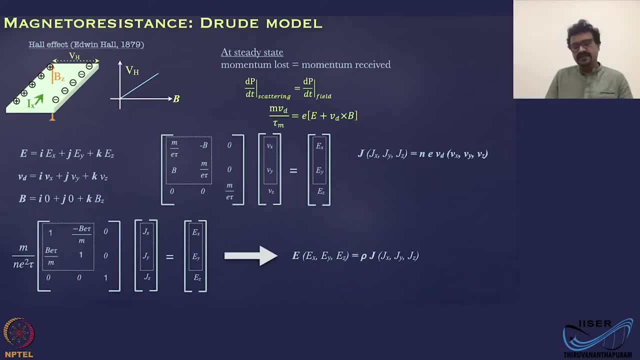 Now what we are doing here is we are going to look into the action in terms of the various components of this field. We have field separate into the x, y and z component, the velocity, the drift velocity, v, x, v, y and v, z, and the v field, which we have played only in one direction. 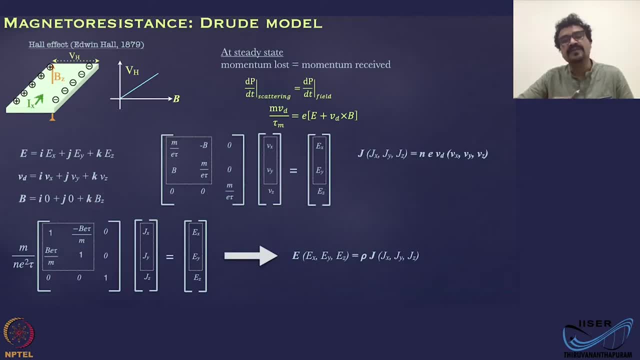 that is the v z. that is the only component I am going to talk about in this lecture. I am going to consider: ok, And once we substitute these three in this equation, you can generate this matrix. ok, So I have marked a small square matrix inside. 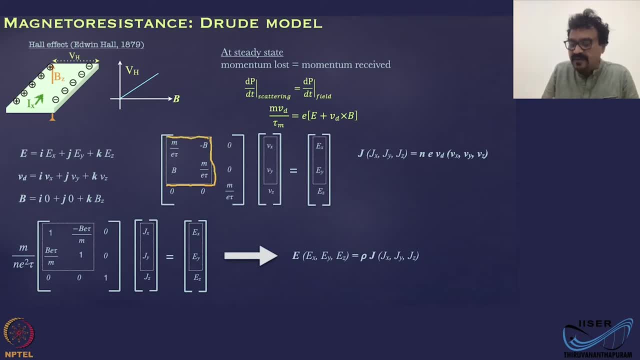 this as 2 by 2 square matrix inside this. that is what is going to be relevant For a two dimensional system eventually. that is what is going to decide the whole voltage and whole effect, because the moment you apply the magnetic field, all the action of electron, 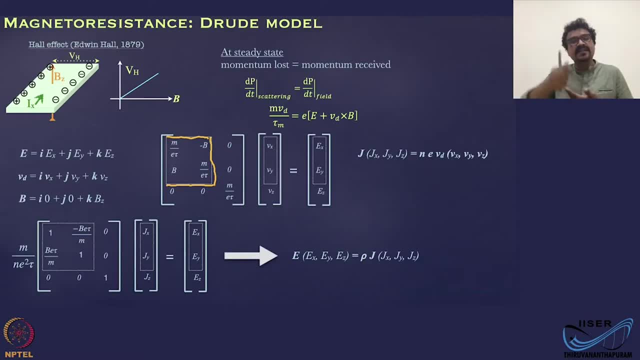 happens in the plane, whereas the direction along the field or parallel field is not going to get affected by the field. So there you will not see an effect of field ok in that component. So when you have asset all, when you substitute these equations into this equation, you will. 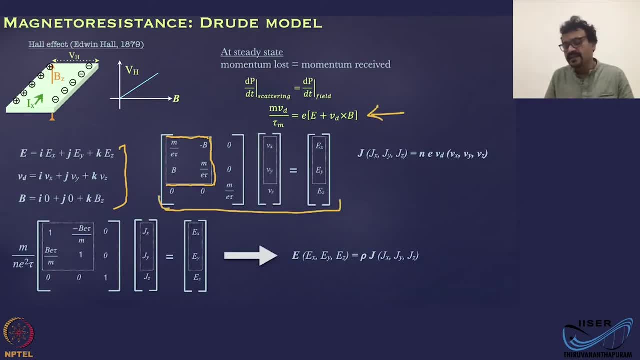 generate this matrix equation and from this matrix equation you can generate this one by substituting j equal to ne into bd IR. J is the our one on in m And for next question, we are going to think about nonvectorization. 제가. 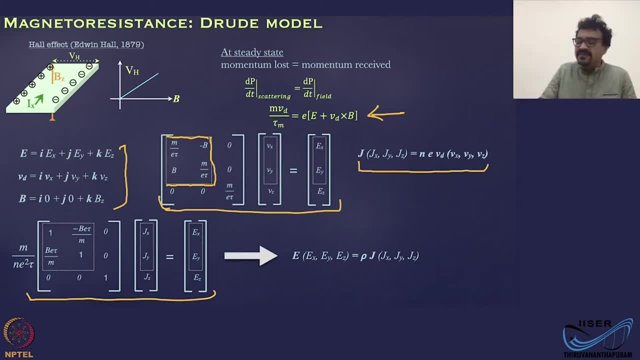 am the one in Chemnока University in field three. that is how we were able toiko n. to is the current density: j has the components jx, jy and jz, and vd has the component vx, vy and bz. okay, so the aim here is we need to replace this with the jx, jy and jz component. 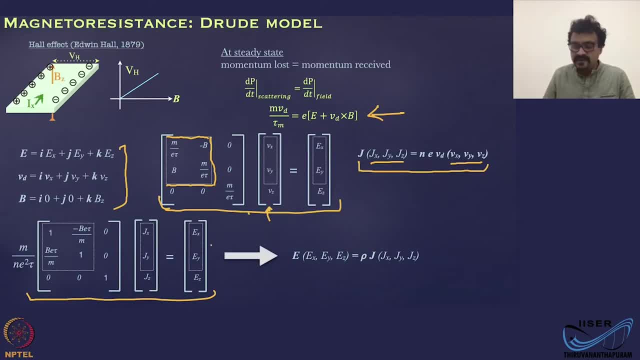 that is only changed when you go from here to here. so here you take this v these and replace those with jx, jy and jz using this equation and you do some rearrangement and eventually you will get m? e square m by n? e square tau. 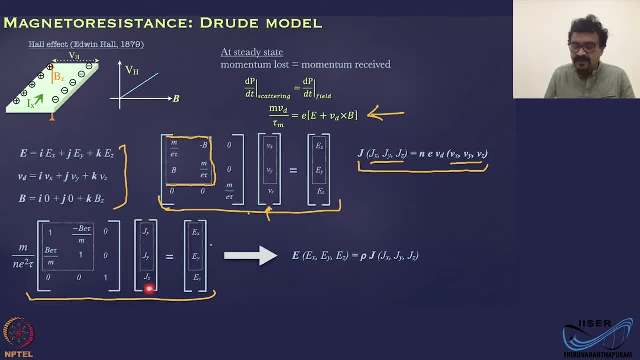 okay, into this matrix. the j matrix is going to give you the j vector, is going to give you the e vector, electric field vector. okay, and this is basically equal to the formulation. e is equal to rho into j, that is the ohm's law. okay, where this rho is nothing but the rest, restivity, j is the current density. 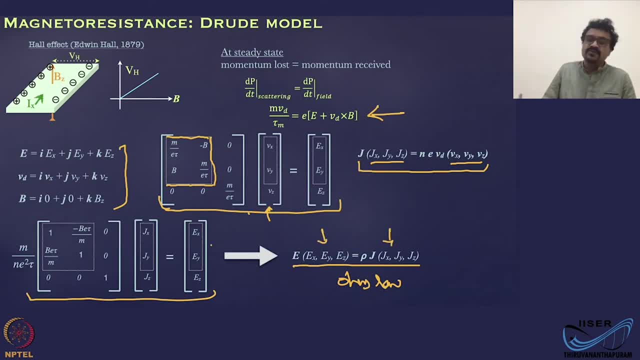 and e is the electric field, because you are familiar with the ohm's law in terms of the um conductivity, but this is just restivity. so what you are familiar with is j sigma into e, okay, and this is just. the sigma is replaced by one, by rho, that's then. you take that row to the other side. 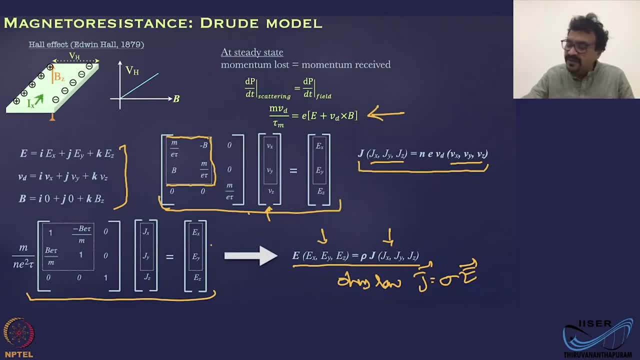 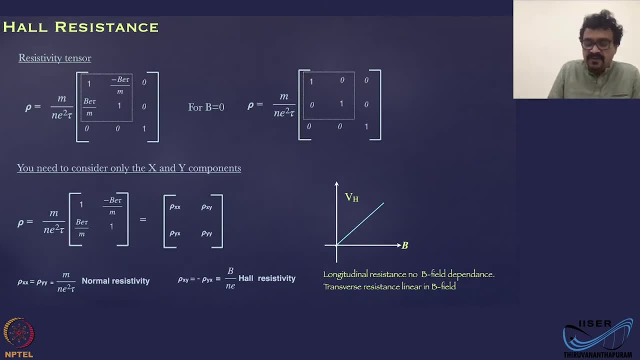 that's what it is, okay. so here, what you have now is you have this row, the resistivity as a tensor. it's a resistivity tensor because it has components in the all in all the direction. okay, so it's a three by three matrix. m is m by n? e square tau. 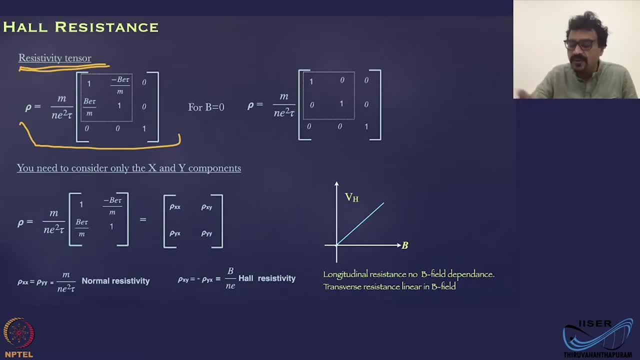 is the restivity when you don't have, you have no b field, or when the b field is zero, and this is an isotropic quantity. when you don't have any b field, the moment you turn on the b field, you're going to get this of diagonal components, okay. 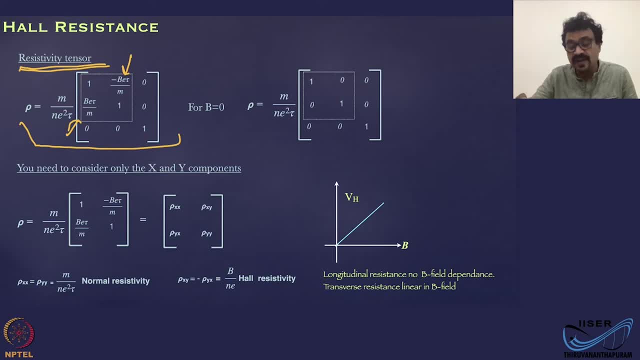 those are proportional to b field of diagonal components, but diagonal ones are independent of of the b field. Now, as I told, the third row and third column, which represents the component which involves the z direction, we do not need to consider because field does not do anything. 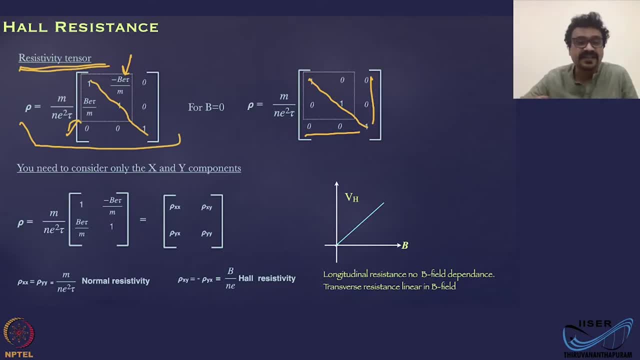 in that direction. the magnetic field does not do anything in that direction to the charge carrier. so for the time being, to ease the discussion, we can ignore that and we can just take the matrix, which is the 2 by 2 matrix here, and that resistivity is given by M, by 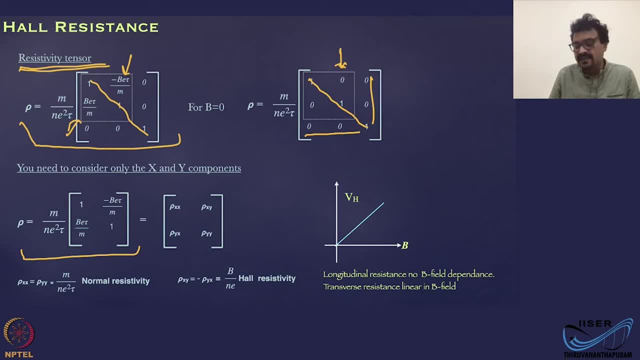 N square tau into this matrix inside and this is of the form you have: rho xx, rho xy, rho yx and rho yy. These rho x y and rho z, rho y x, the off diagonal components, which involves magnetic field and the diagonal components. 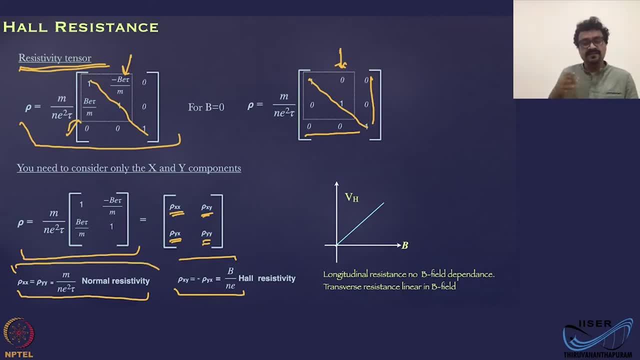 which are your normal resistivity, which is equivalent to the your Ohm's law derivation using the classical Drude's theorem, This is normal resistivity, and the off diagonal components the rho x, y and rho y x. the rho x- y is negative of rho y x is b by n e that 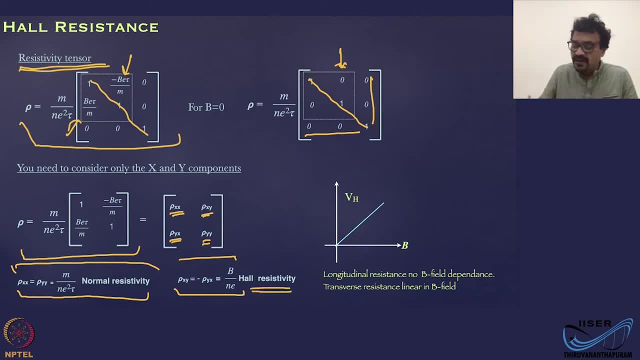 is the Hall resistivity. ok, And the Hall resistivity is proportional to b and it is inversely proportional to n. So directly from this slope you can calculate the carrier concentration from here. this is proportional, the Hall resistivity. So v, h by i, that will give you the r, rho, x, y. ok, that is your Hall resistance. ok Now. 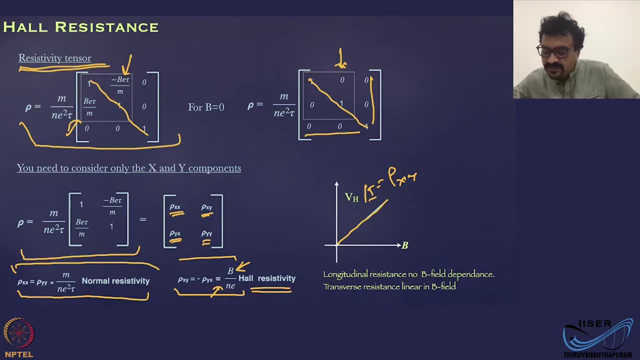 that is proportional, that the slope of that is proportional to the b field, ok, But at the same time the longitudinal resistance does not have any dependence on the b, Whereas only the transfer resistance is proportional to the b field. ok, So this is proportional. 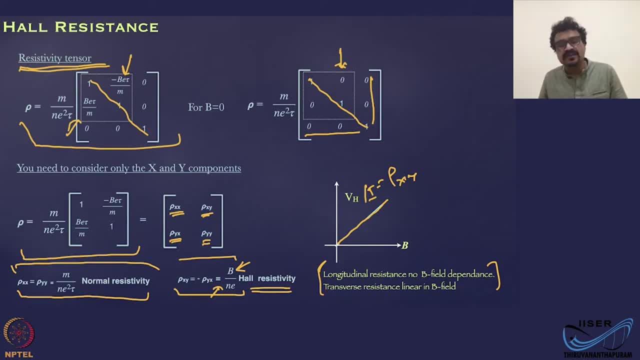 resistance as a dependence. Longitudinal resistance is the resistance along the propagation, along the direction of the applied electric field, and transverse is the one which is normal. perpendicular to that is the x- y term If we assume the electric field at the x direction. 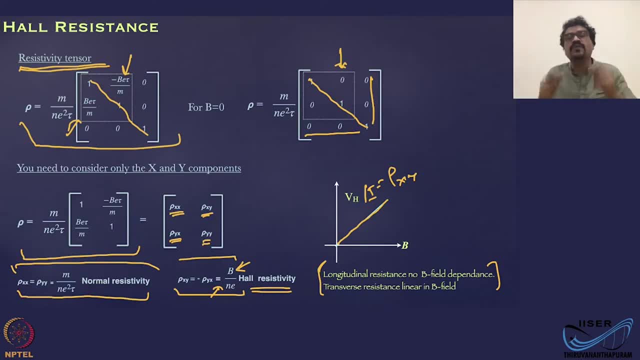 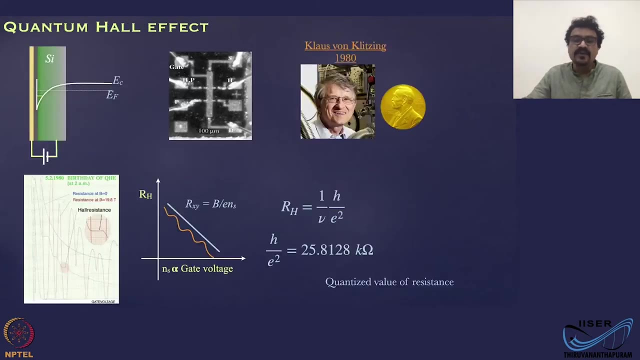 magnetic field is a direction I am discussing, or I am talking about x? y direction, The x y direction that is proportional to the b field, and this is the classical Hall resistivity. So this is the classical Hall effect. alright, Now, if you do this experiment, the same Hall. 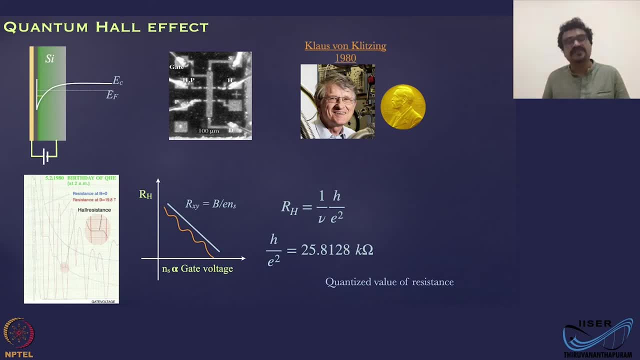 effect experiment in a two dimensional system, a clean two dimensional system, ok. When I say clean two dimensional system, just ample mean free path So that the electrons which are undergoing the cyclotron motion can complete the full. I mean full, full circle, at least one full circle, ok. Now if you do this experiment in 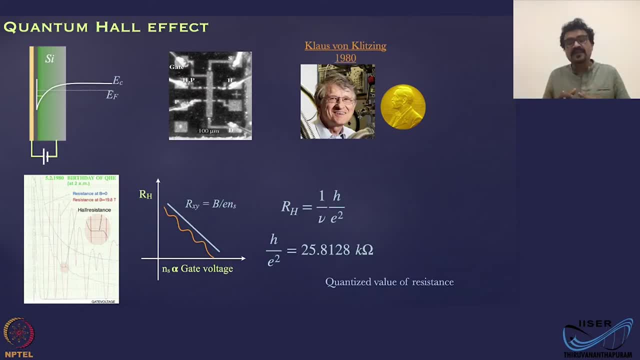 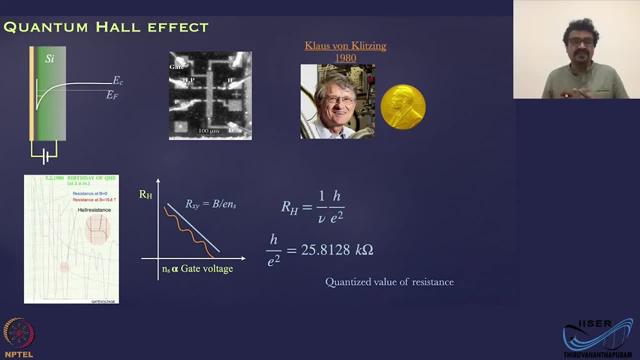 one full circle, at least one full circle. Now, if we observe this in a normal system, it is going to be a slightly different Hall effect picture. So that is the quantum Hall effect. ok, That's a, that is a quantum mechanical counterpart of the Hall effect. ok, So I will briefly review. I will give you an all view. 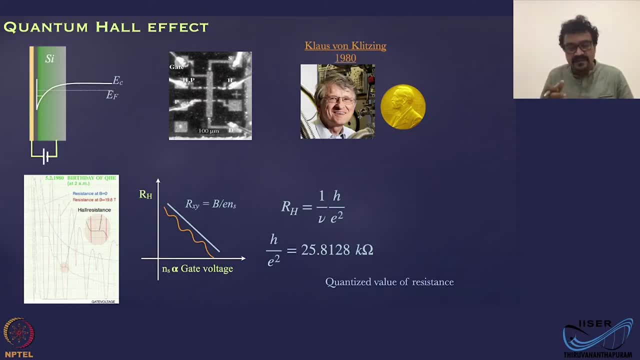 of what that effect is in this class. Now, how that effect is in this class, I am showing How that effect is used in certain technology is called the quantum electrical metrology. in quantum electrical metrology, as a resistance, universal resistance standard, The quantum Hall effect was discovered by Klaus Wolclitze in 1980, which earned him the 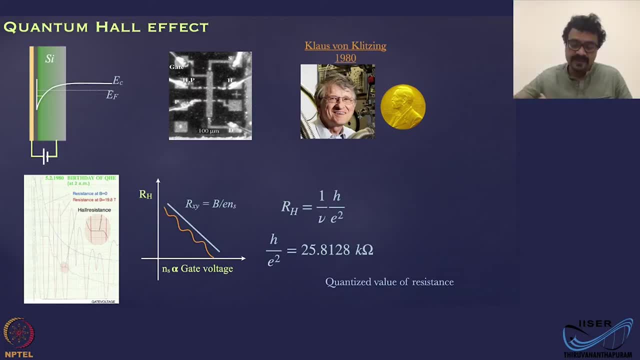 Nobel Prize. So this is an extract from his lab notebook, von Kleinstein lab notebook, which is the birth of the quantum Hall effect. So here what we have is a silicon dioxide and metal. that is a some. it is a MOSFET and this is the top view of the MOSFET, which is 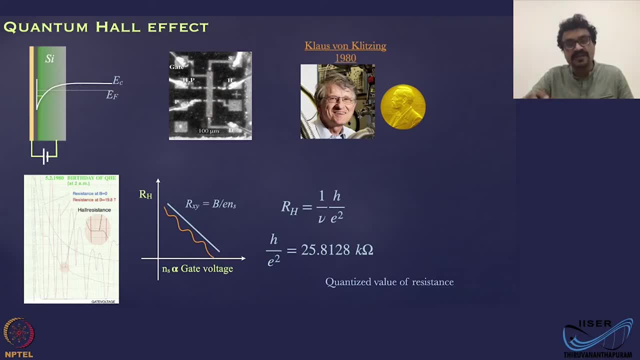 a classical. So, for the time being, what you can assume is you have electrons or you have charge carriers. wherever you are seeing these lines or these bright regions, those, those are the basically gates you can take. ok, where you have carriers in those regions, ok, So what do you have? 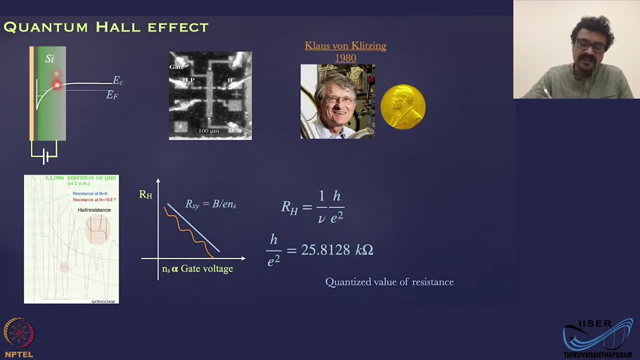 is when you apply voltage onto the gate and you have a silicon substrate. it is a MOSFET. you are going to create a thin accumulation layer which looks like a quantum well, Which is actually a quantum well, triangular shape, quantum well. at the interface You have charge. 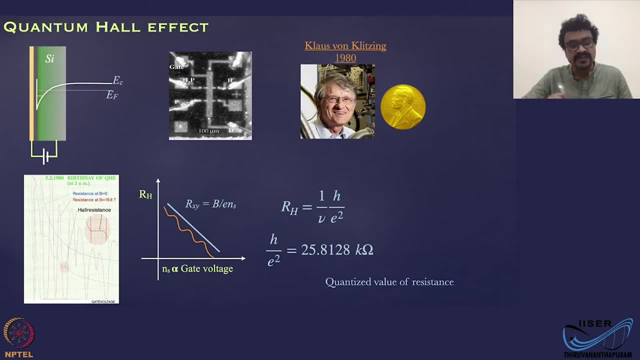 carriers here. this is low-energy region for electrons. the Fermi level is somewhere here and you have a triangular well and the well thickness or the width of the well is such that we have only one quantum level populated below the Fermi level. That is actually a two dimensional system that is very dense and a hole is not greater. Then in this case there is a increase in battery, I mean pressure like a lot. and this is the phase field of the site of the first 1 to 2제를, maybe 1 to 2 mình ollut phase. that is actually a two-dimensional. 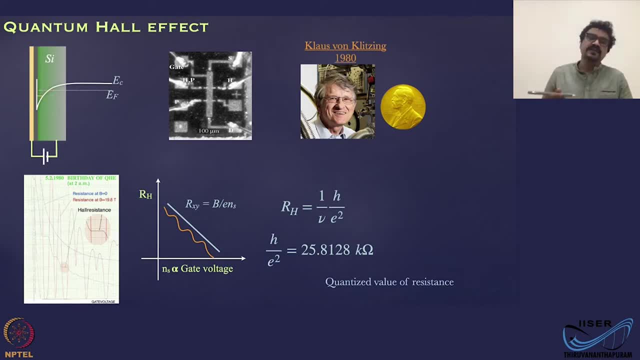 dimensional system where the, in the world, in the direction, in the z direction, which is perpendicular the plane of this substrate, you have only one momentum state or there is only one k state. so then you can assume that that's a two-dimensional system. okay, but the charge? 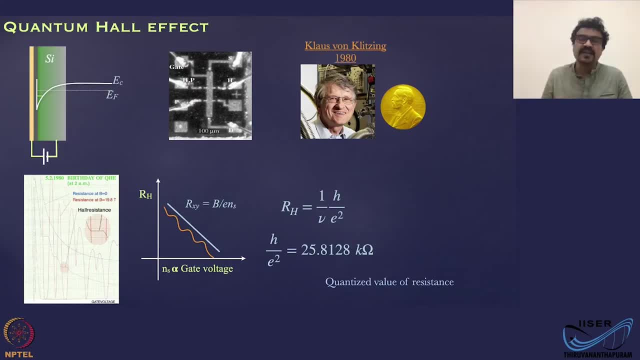 carriers, as we discussed in the gallium arsenide- aluminum- gallium arsenide four-dimensional system, the charge carriers are free to move in the plane, but decorate move. there is no momentum state available for the charge carriers to scatter in the either direction. okay, now the experiment is as follows: you have a b field which is applied perpendicular to 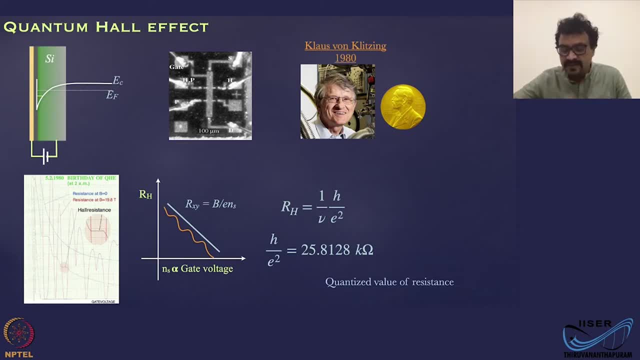 sample perpendicular to this material. then what you do is you vary the gate voltage which will change the charge density for carrier conservation in this step. okay, so you have, you have carriers in this, well, and you are going to going to change the that carrier conservation which i have labeled. 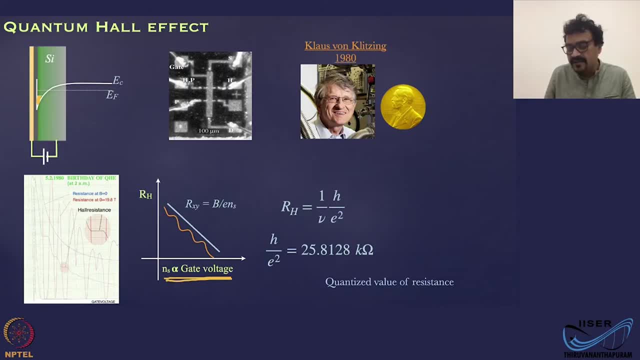 ns, which is linearly related to the gate voltage. it's a capital thing. it's like a capacitor, but you are applying a voltage on this capacitor plate and the second plate of the capacitor is the two-dimensional electron system. so the number of electrons, which is the charge q on the capacitor plate, 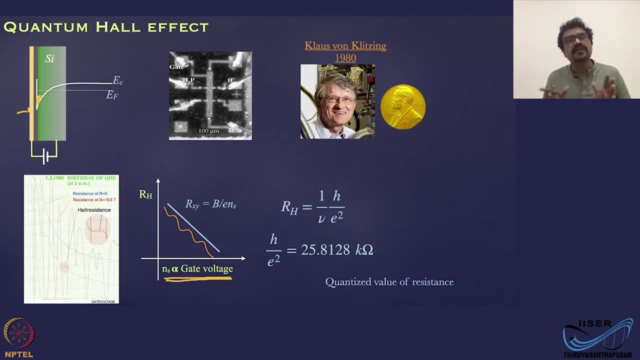 is basically proportional to the voltage on the capacitor plate. okay, that is the gate voltage. now, usually, as far as hall effect is concerned, the classical hall effect is constant until this phenomena was discovered. you have rxy. is b by e and n, is it that means when you vary the carrier? 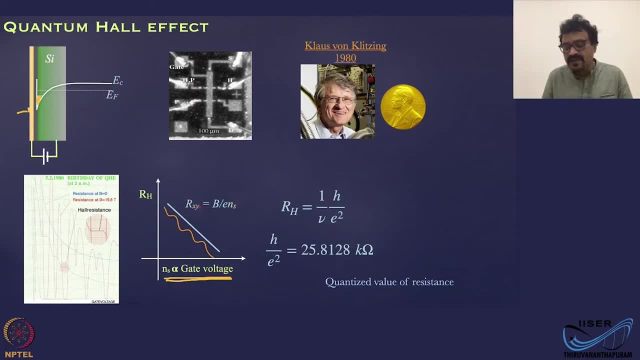 by the gate voltage that there should there should be a reduction in the rxy, which is the rx, the whole persistence. so what is expected as per classical physics is this linear shaped straight line. okay, it's a straight line. now what was observed is something like this: so if you look this, 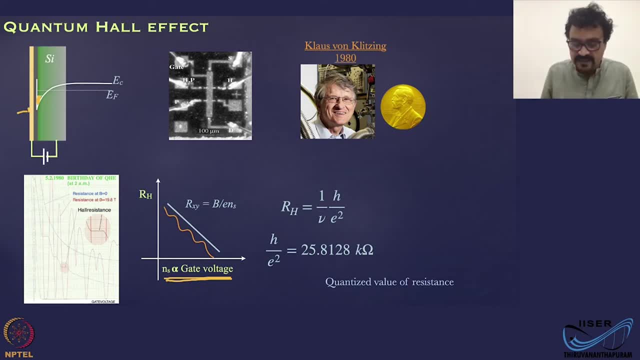 uh, graph carefully, let us focus on this curve. so if you look this graph carefully, let us focus on this curve. let me try to draw on top of it. so this one when you have step region, another step under step, this curve, okay, so i have kind of try to give you a feeling of what the curve is going to look like. do you have? 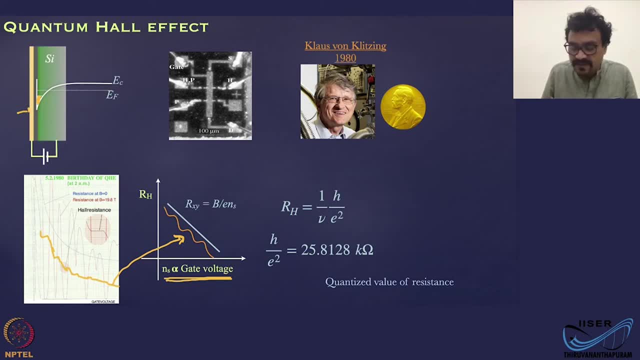 flat. we have step shaped curve and this is a magnified view from that curve. okay, so you have a flat region. it's a step as quantized certain value rx, which are given by this formula, where nu is an integer. okay, so what we have is you have a step shape curve instead of 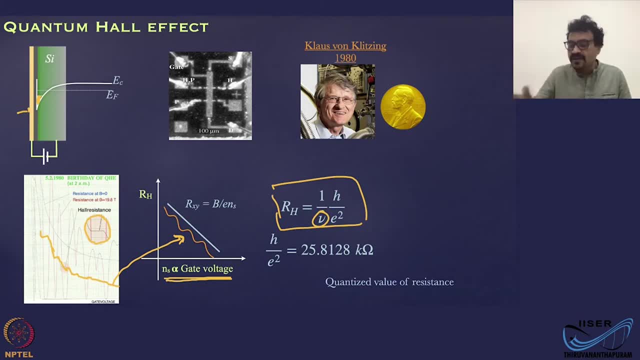 a straight line where the step values are actually quantized in h by e squared. that means the the highest value is h by e square and the other steps are one by nu of h by e squared. okay, for h by e square is the resistance quantum or quantized resistance value, which is equal to 25.8128 kilo. 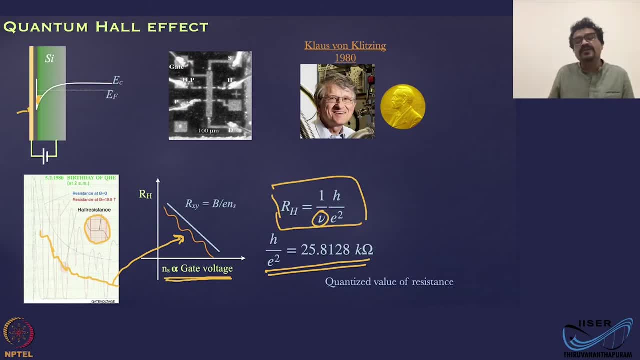 okay. so this is the quantum hall effort where the all resistance is quantized in h by e square. i would say conductance is quantized because all resistance is one by nu where nu is an integer. okay, you say integer okay. so it is rhs quantized in one by nu where nu is in this into h by e square, okay. 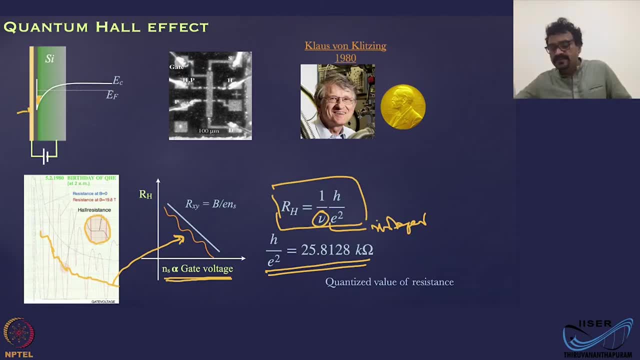 this is the quantum heart. now, this was done in silicon, mosfet geometry in silicon, at low temperature, okay, so you can see that this is done at really high field, okay. and even what time is also marked: it's around 2 am, you know, early in the morning, okay, which earned him. 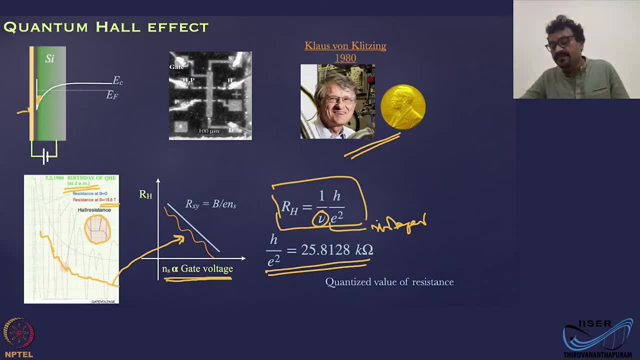 the number place in double place in physics. okay, this discovery happened in 1980.. now what we have from the previous slide is we are varying the rxy by varying ns, but instead of that you can also vary b field, the magnetic field. so the later generation, high mobility, generation of. 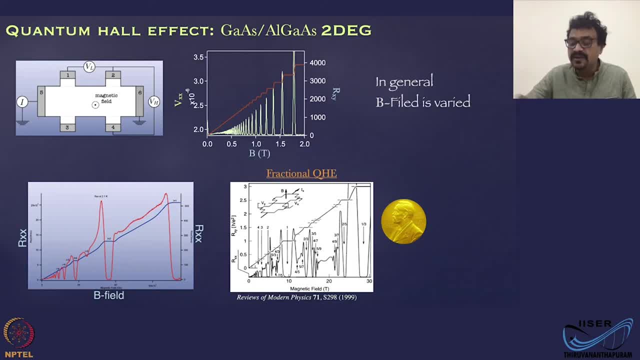 high mobility material based on the, the three, five, the gallium arsenide, aluminum gallium arsenide or similar system. those are remotely dropped. they already have carriers in the well, in the quantum well. the formation of the well we have discussed extensively in one of those modules. okay, so you? 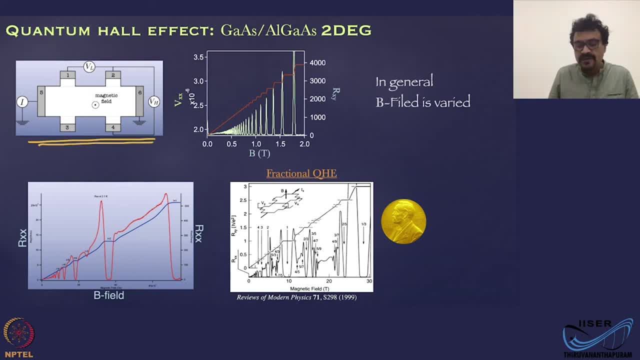 have again similar geometry, where you are injecting current and you are measuring the voltage across or perpendicular direction of current. where is the where the magnetic field b is applied- perpendicular plane- okay, and this data is taken using one of those samples and what you are seeing here is the rxy. 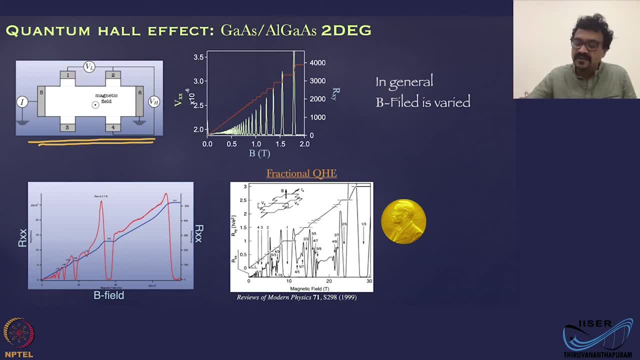 the whole resistance is showing a step-like feature, as shown here. okay, this rxy. okay. now, at the same time, you are also seeing a vxx, the voltage along the x direction which is measured across one of these probes in the direction of the current propagation. okay, and that is also showing oscillation. okay, 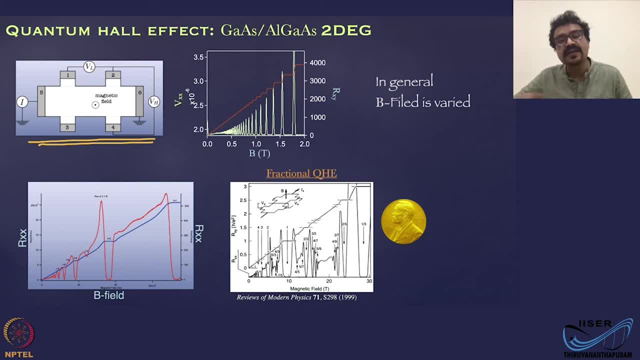 so this oscillation in the current, in the direction of the field, is called sobrikoff d, has oscillations and this is the quantum hall effect, the step-like feature in the rxy, and you can see this is one of the high field behavior. here is the low field behavior. okay, the high field behavior. you can see that you have plateau at. 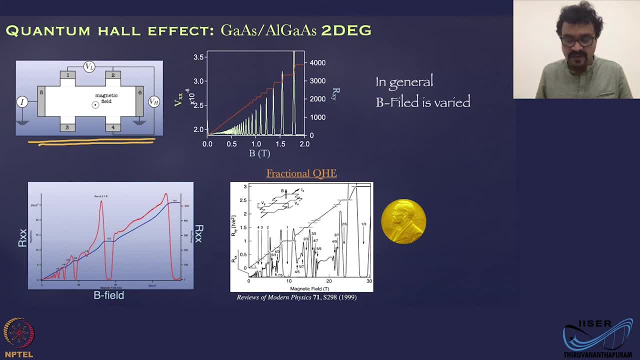 that you know any single loop one, this axis you have to map back to here. this is the axis that is around 25, point. no, it's not around, it's actually exactly 25.8138. and the second one is here, half of it, and third one is here, and so on. okay, and 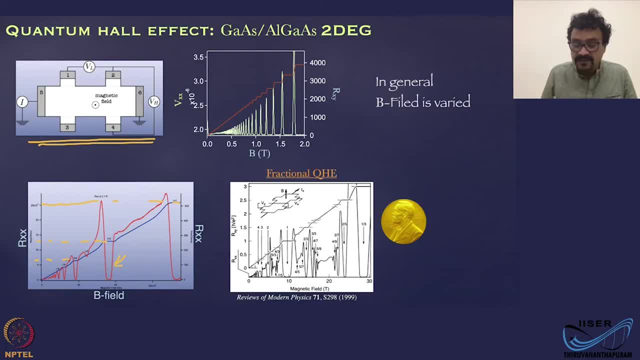 there are also oscillations: the red shaped, red colored curve in the rxx. that is a linear resistance, resistance along the direction of the field. so if i mark it here, r, x, y will be this and rxx will be the resistance in this direction. okay, the direction. 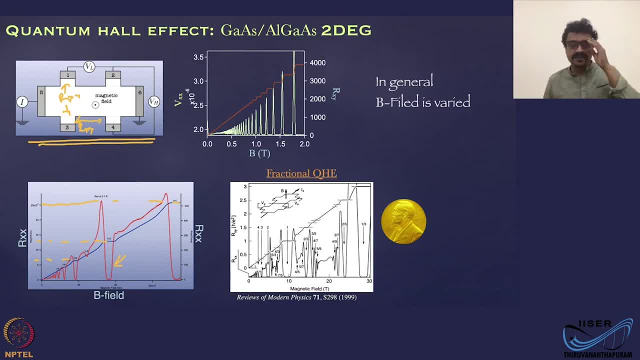 in the direction of the field- electric field. okay, now let's look at the rxx field. a few years later, as the technology of making higher and higher mobility material got matured, the experience start observing a slightly complicated, intricate hall effect that is called fractional quantum hall effect. okay, in this case, 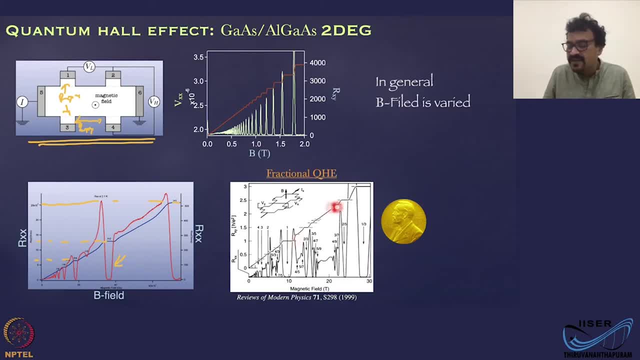 you have plateaus or flat regions in the rxy, but not only at integer values but also various fractional values as mark here. this, if time permits, we will try to dis. you will discuss in one of the classes, but this is not going to be discussed in detail anyway in this. 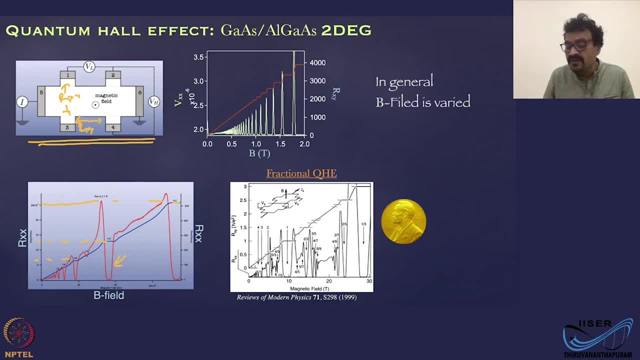 course, just beyond the scope of this course, okay, but this is called fractional quantum object, where you have president's contest at fractional де values. certain fractional values- one, one, third, two, fifth, you know seven, third, you know nine, fourth, and all these values, okay, which are marked here, that earned a second noble price for the. 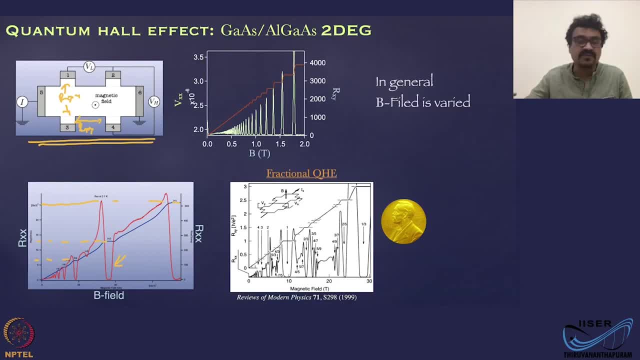 quantum hall effect phenomena. okay, the first one was for integer quantum hall effect, the second one was for the fractional quantum hall effect, and this is a very fascinating phenomena whose physics is kind of very different from that of the integer quantum hall effect. so, to put it briefly, integer quantum hall effect is something which 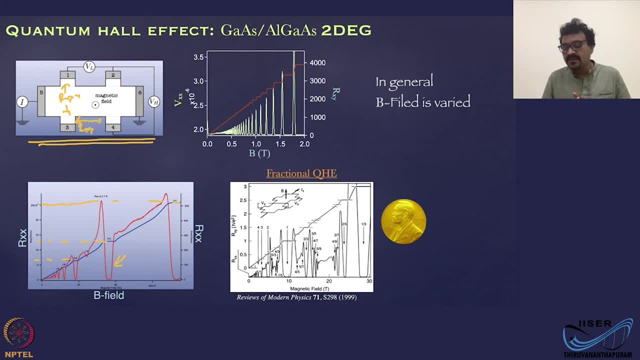 you can explain using single particle picture. but fractional quantum hall effect is a many body phenomenon. okay, there are fractional states, there are composite particles. here you have electrons, but in this case you have composite particles. okay, so that is a anybody. there is a many body phenomena, but of this one you can explain with the single particle. 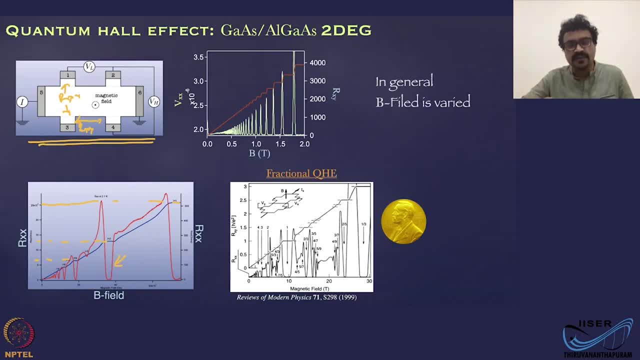 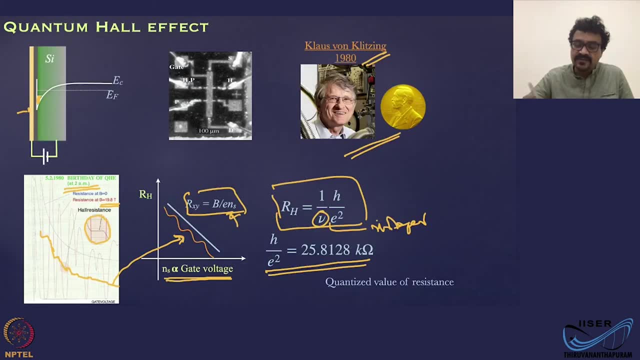 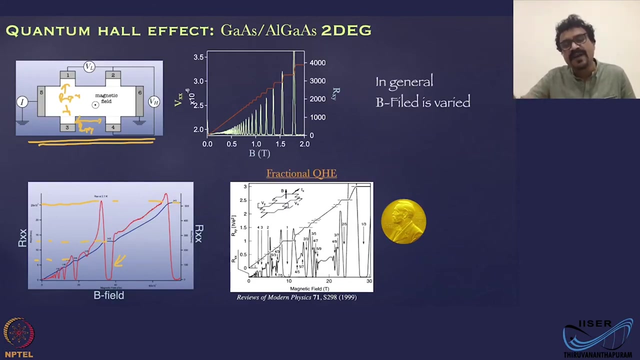 picture. okay, and that we will explain during this course. okay now, the difference here is: in this case we have varied the carry concentration by fixing the b field. in this case, we have fixed the carry concentration but varied the b field. but anyway, the ratio between the magnetic field and the carry concentration is what we have varied. okay now, 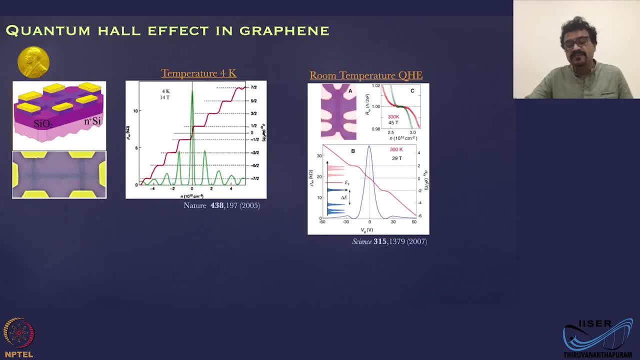 the advent of the new generation two-dimensional systems, the first one being the graphene. it is a sheet of carbon atom and one of the first experiment after extraction of a sheet of carbon atom of after extraction of sheet of carbon from graphite, is the magneto transport, where you apply a magnetic field perpendicular plane of the sheet, where you 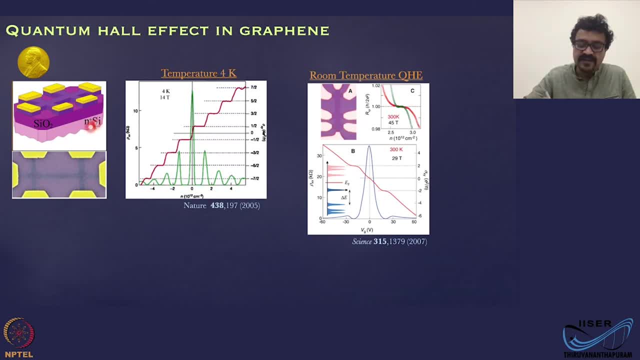 have a back gate which is highly doped silicon, and there is a silicon dioxide gate oxide. then you have the sheet of graphene. then is patterned to form in the form of a hall bar. this is the top top of the sheet of carbon atom. so that is a basic overview of that. okay, and when you conduct the 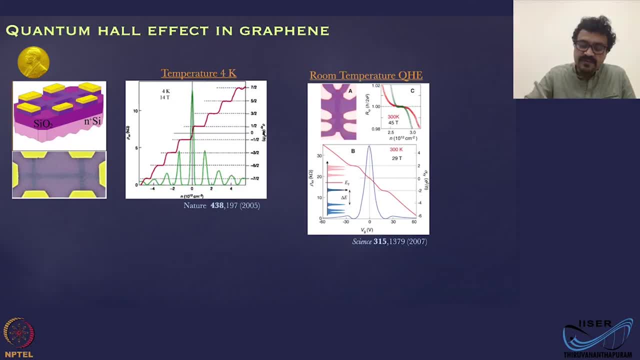 same experiment where you measure the transfers resistance as a function of magnetic field over carrier concentration. so in this case the magnetic field was fixed at 14 tesla and the carrier concentration was very by varying the gate, the back gate. okay, experiment was done. then also they observed a step-like feature as opposed to a straight line. 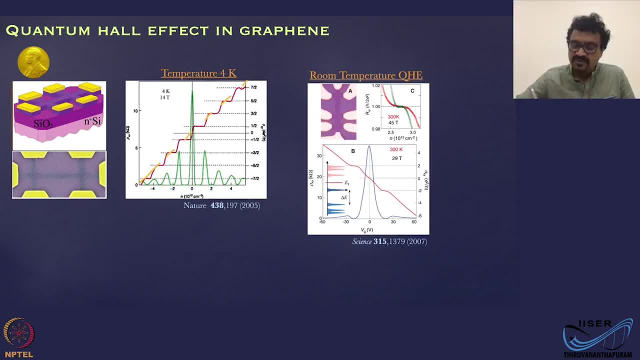 in the hot effect and of course they also observed oscillation in the rxx. that is the green color here. this experiment was done at four color. okay now, this red colored trace represents the whole resistance and that also shows step-like feature and is quantized, if you look at carefully. 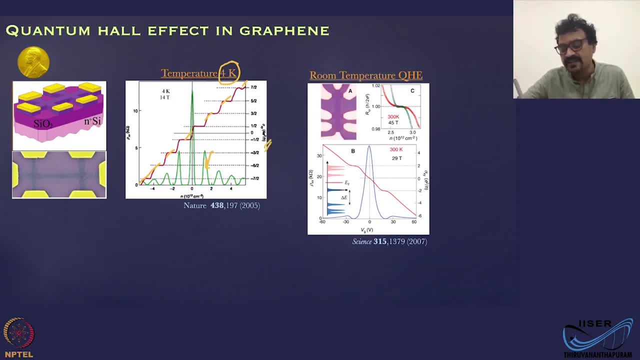 the unit here is 4 e square by h. okay, instead of e square by h. and the detailed physics, if time permits, we will discuss. but that has to do with the nature of this charge carriers. those are not the normal conduction and electrons that you find in. 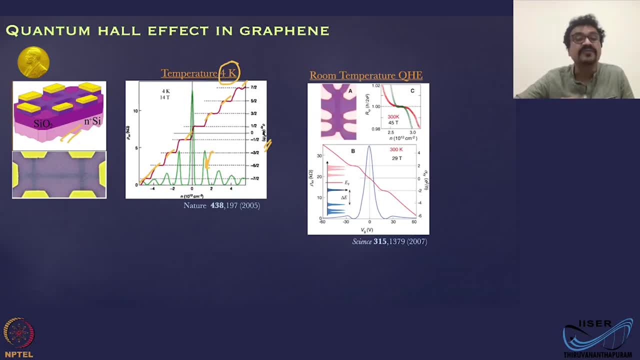 these kind of free electron gas, the silicon electron silicon or gallium austenite material. here you have a drag particle, massless fermions, and you have valleys and you have spin degeneracy. that all these, because this is done at a really high field, all these together. 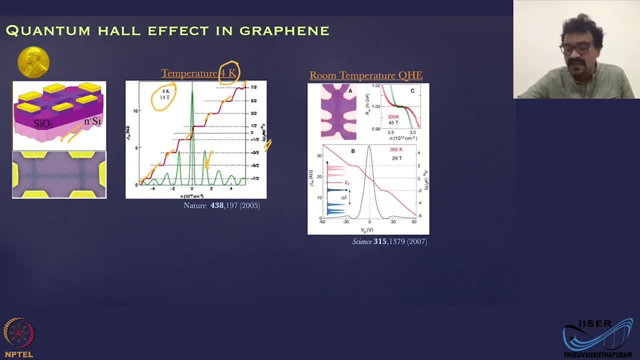 is going to form a free electron gas and a material which is going to have this free electron gas and all these, because this is done at a really high field. all this together is going to go very, very well. going to give you a slightly different Hall effect, but still it is quantized, the resistance. 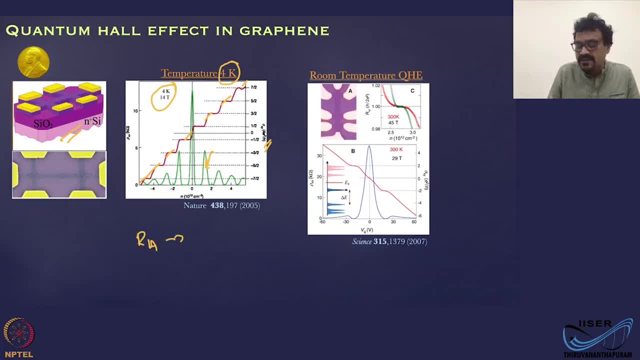 is Hall resistance. RH is quantized. that is the point is quantized in this picture also And surprisingly, this effect was observed even at room temperature. ok, You can find more details about these in these 2 papers. ok, And I would say that is probably I can. 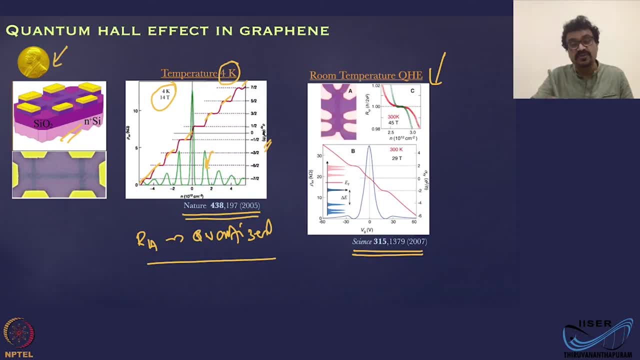 say this is the 3rd Nobel Prize for quantum. it is, though it is not directly for quantum Hall effect, but the feature that demonstrate in this experiment is the quantum Hall effect. ok, It is probably the 3rd Nobel Prize for performing a quantum Hall effect experiment. 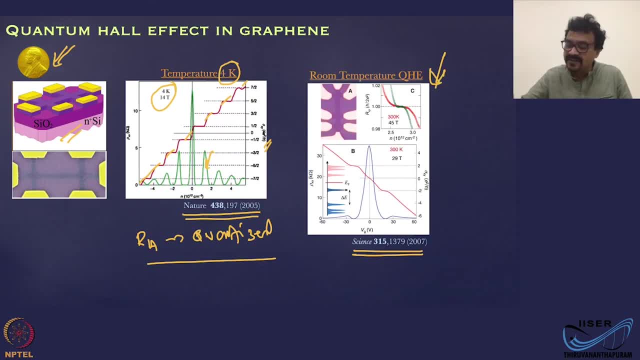 And we shall see more details in these 2 papers. And, interestingly, you can see these quantization even at 300 Kelvin room temperature in a sheet of graphene. That is awesome, okay, So what we have now is: you have seen this effect. 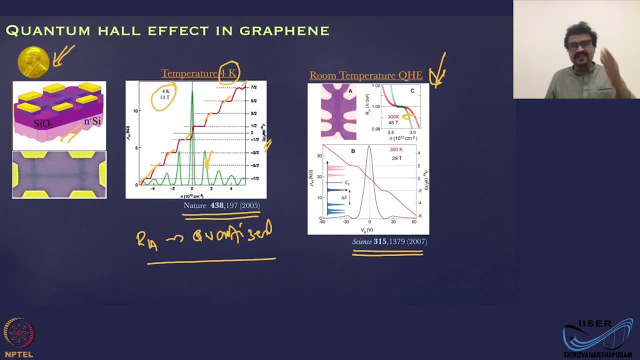 in, starting from a silicon MOSFET, then you move on to gallium arsenide structure two-dimensional electron system. They're also using the same effect. And now there's another completely different two-dimensional system. It is radically different. Those are bulk two-dimensional system. 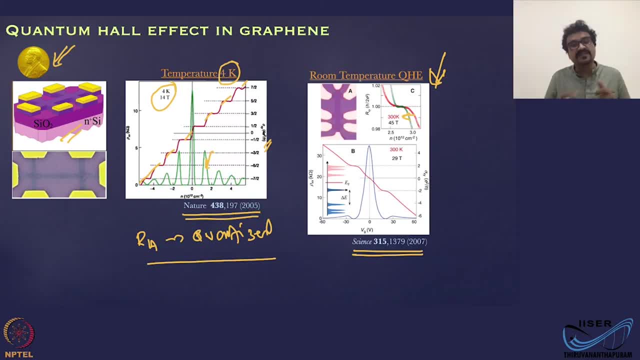 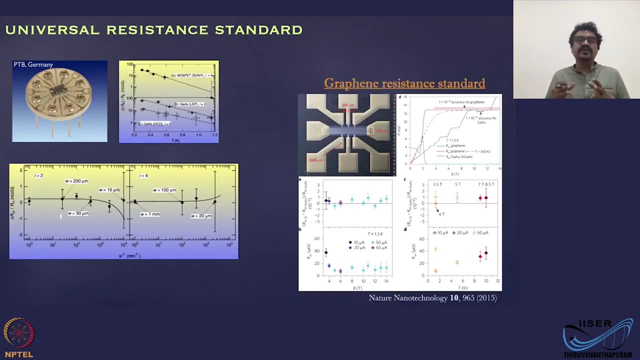 or interface in the bulk material, the first two ones, But this is actually a sheet, a pure sheet of atoms. There also you are seeing the same effect, the quantization, And it's so robust. So what we now have to do is: 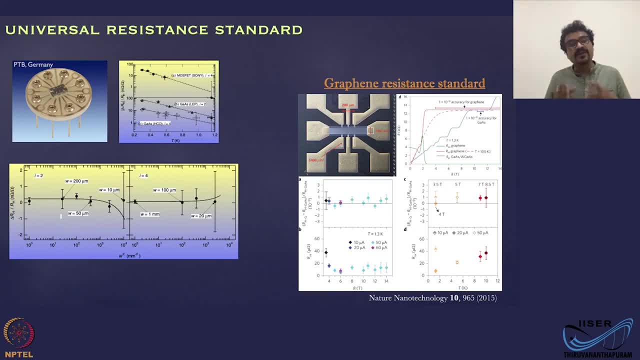 what we now need to realize is this: quantum Hall effect is a universal phenomenon. It doesn't depend on material system- okay. It doesn't depend on the kind of equipment you use. It doesn't depend on the temperature, As long as certain energy scales are met. 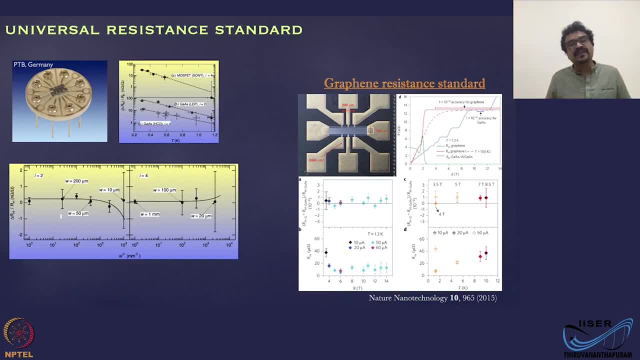 you will see this effect. So, and this was initially proposed and now this has been widely well accepted and followed as a resistance standard, universal resistance standard in quantum electrical metrology. So this is a picture of one of those samples. It's a gallium arsenide sample. 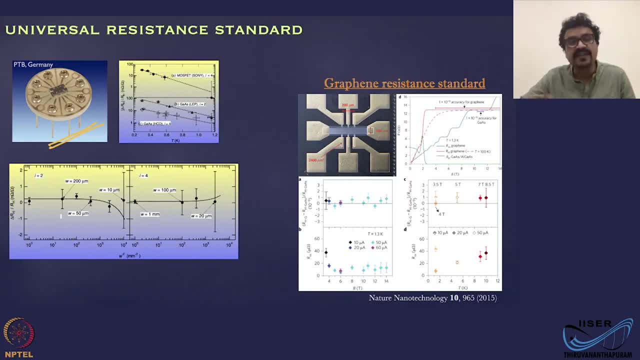 but this has been done on various materials and verified across the world, across the countries. that is such a robust phenomena And the plots. here are the three elements. There are two atoms out of the carbon errors that are measured in this context: values over systems. those are in nano. 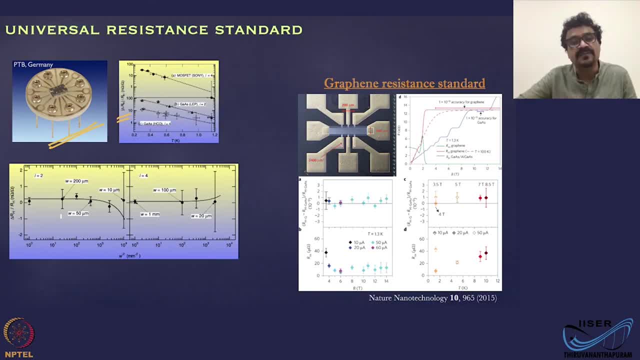 ohms. okay, at 9 place after the December. okay, all these are in nano ohms if you read the axis carefully. these are all error. that has been their variation. that has been measured over various systems. this is not even like one nano okay one. this will scale. here is like three or four arose, okay, now in this case, okay. so 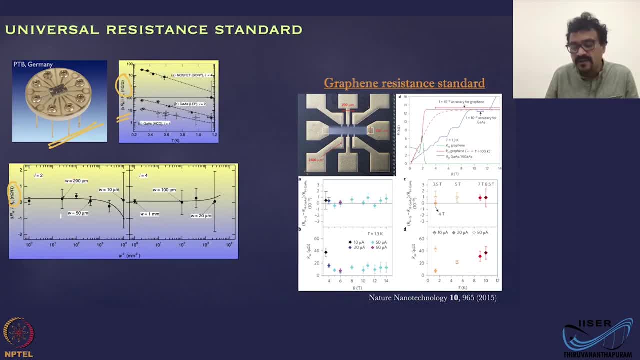 here is a 200 micro meter-wide device. this is like 50 micro meters is a 10 micro meter? okay, and it is how the eye is equal to. the second plateau was possession and error between various devices. here this is also this, the fourth plateau, we're. 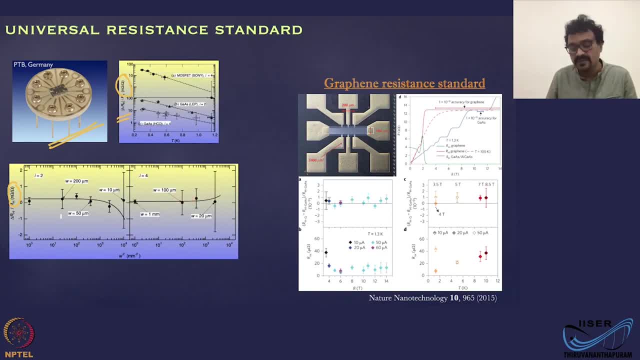 error across various devices is in nano ohms. okay, similarly, here these are done for various materials like gallium, arsenide, as by various labs, and that is their error bar, overall error bar across all the device. okay, that is in nano ohms. that is nine place after the decimal. such